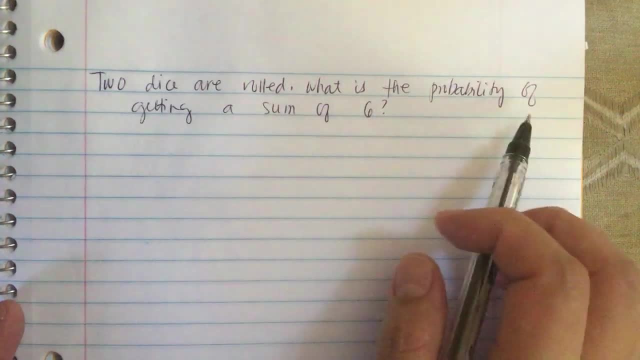 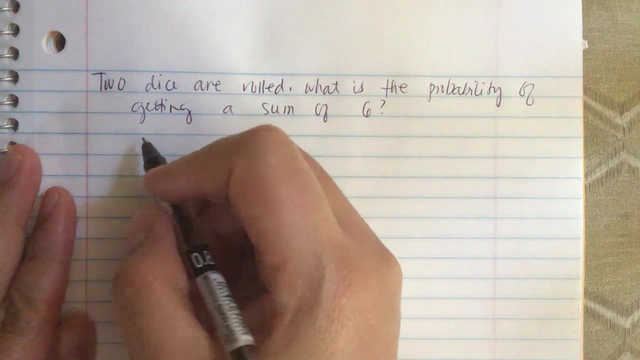 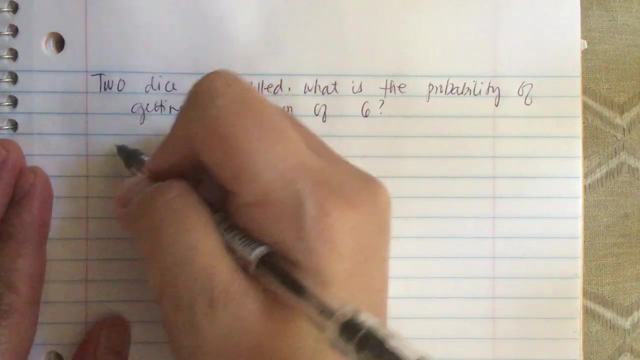 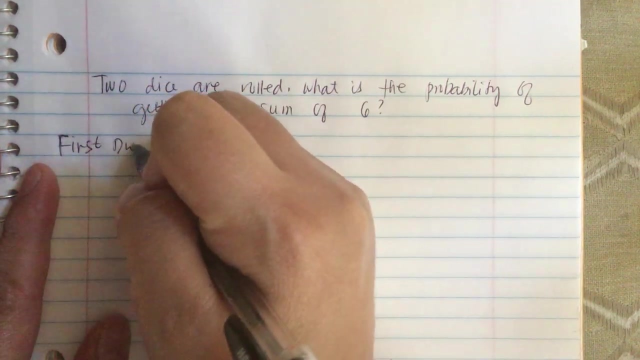 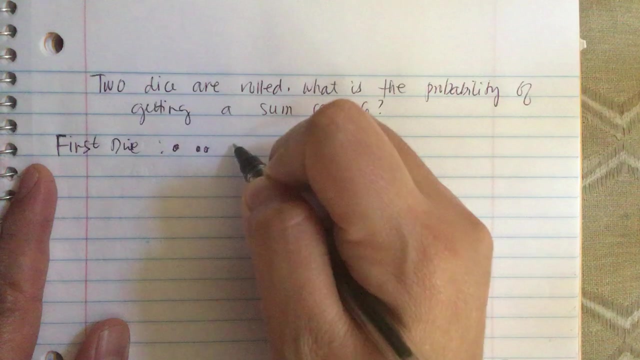 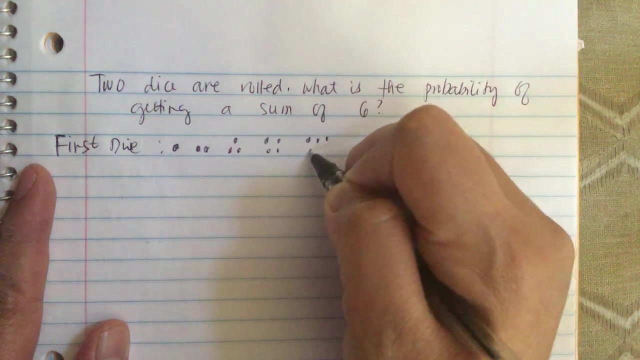 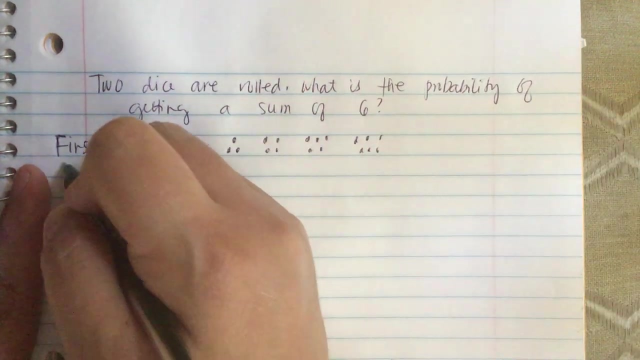 Two dice are rolled, What is the probability of getting a sum of six? So there are two dice, So dice have six faces, So we have, and it is numbered from one to six. So here's the first die, So first die. So we have one, one dot and then two dots, and then three dots, and then four dots, and then five dots and then six dots, and the second die. 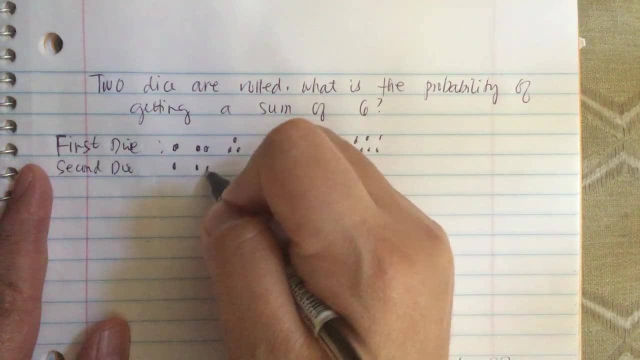 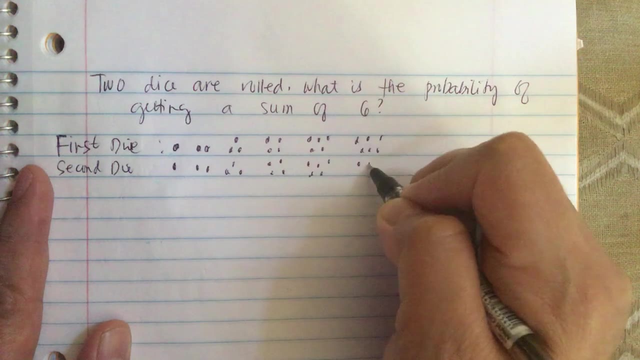 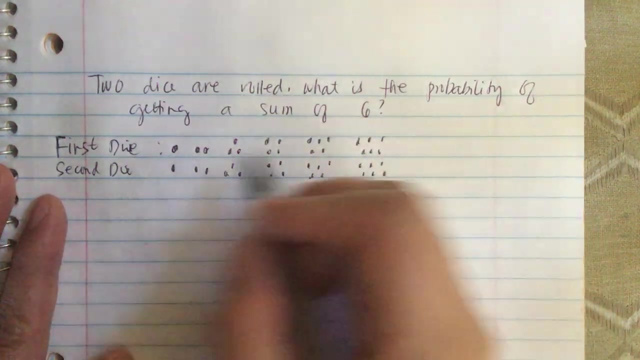 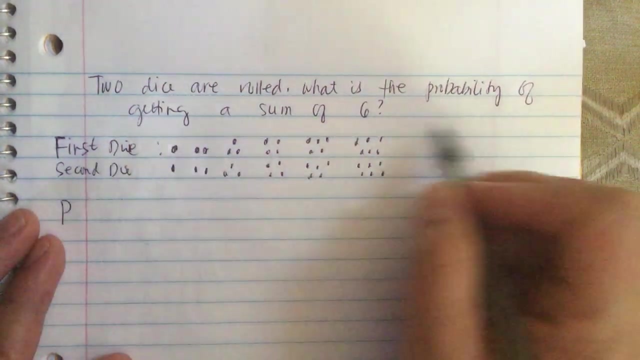 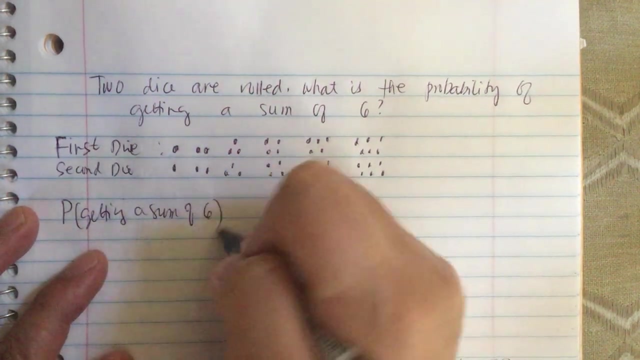 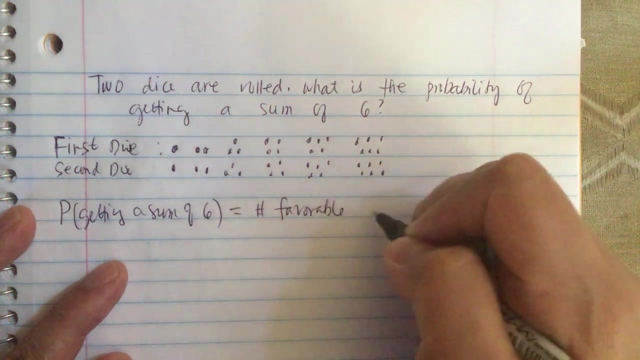 Okay, So this is the second die. So six times six is equal to 36.. So the total, so probability of getting a sum of six of six, is equal to the number of favorable cases on top over the number of total cases. 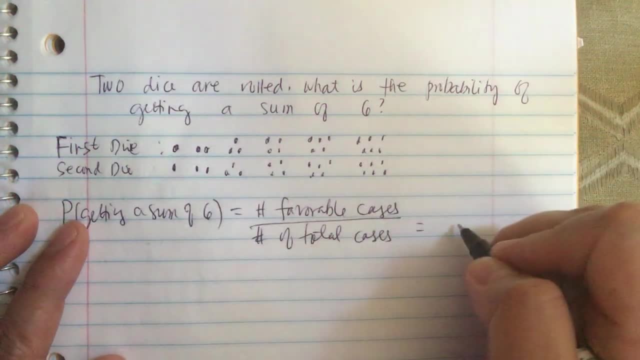 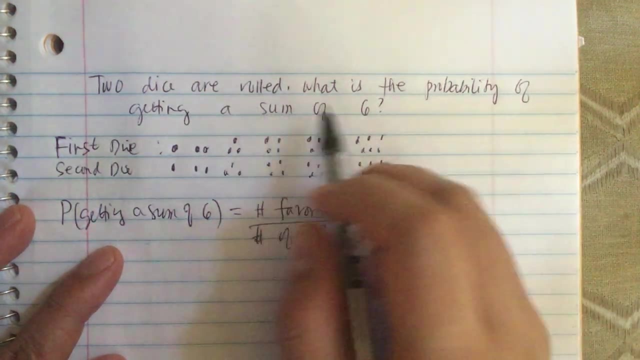 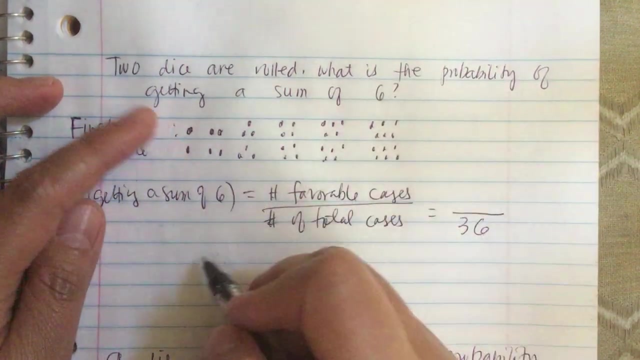 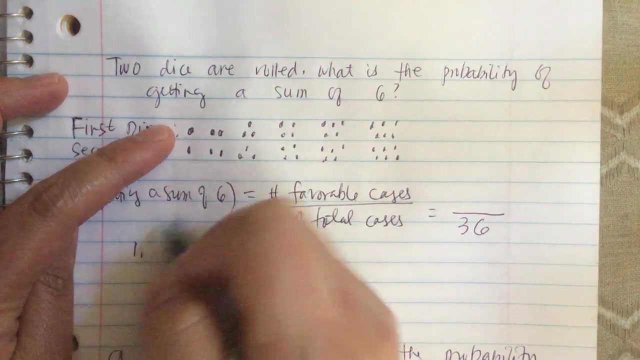 So since there are two dice, so six times six is equal to 36.. So this is the number of total cases. Now the favorable cases sum of six. So let's list all the possible cases. So if the first die is one, then and the second die is a five, So that's a six, So a one and a five. 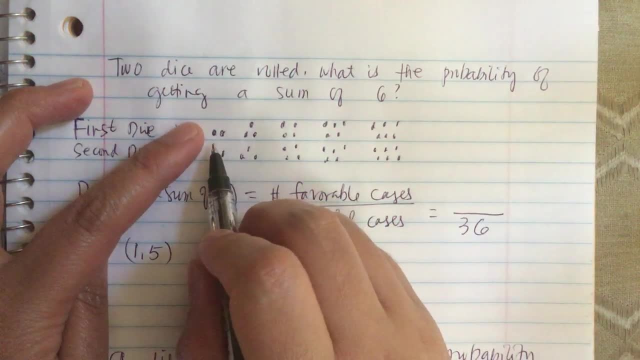 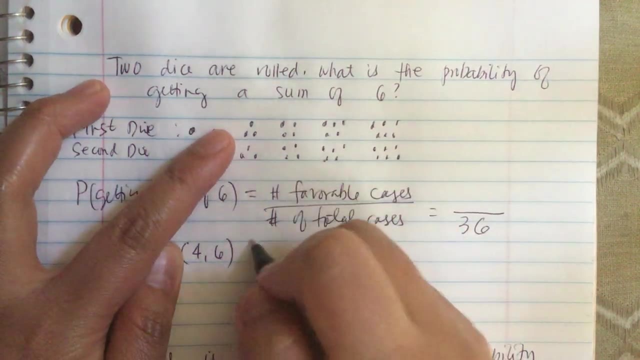 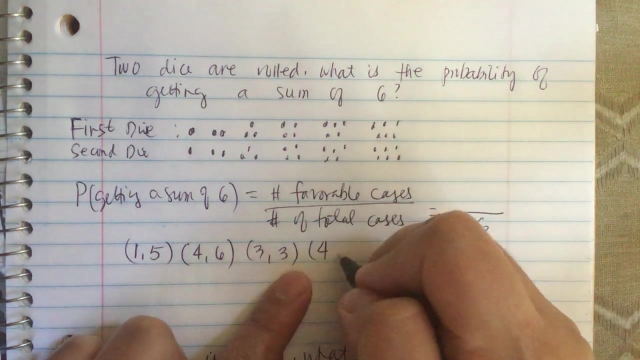 So that's, that's a possibility. So, and then a two and a four is also a possibility. So four and a six, And then we have three on the first die and three on the second die, And then four on the first die and a two on the second die. 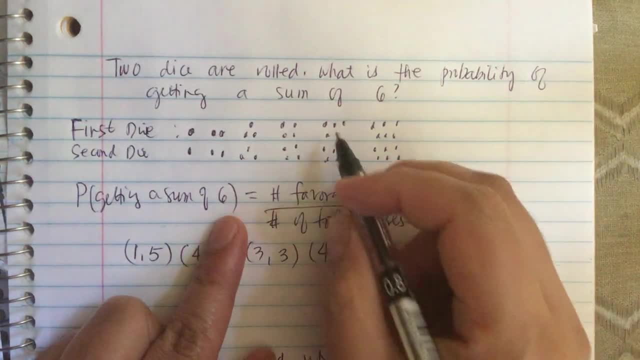 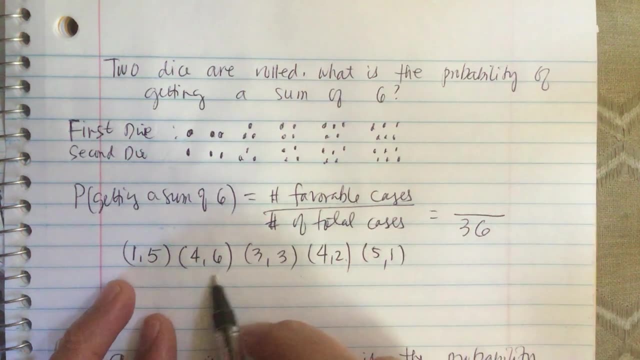 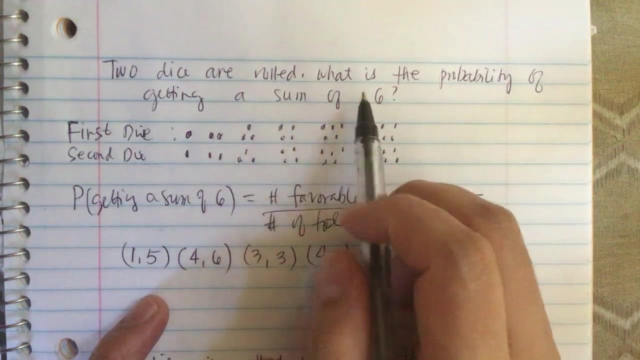 And then a five on the first die and one on the second die. So one, two, three, four, five. So total number of favorable cases is equal to one, two, three, four, five. So the probability of getting a sum of six when two dice are rolled is equal to six. So that's a six. So the probability of getting a sum of six when two dice are rolled is equal to six.